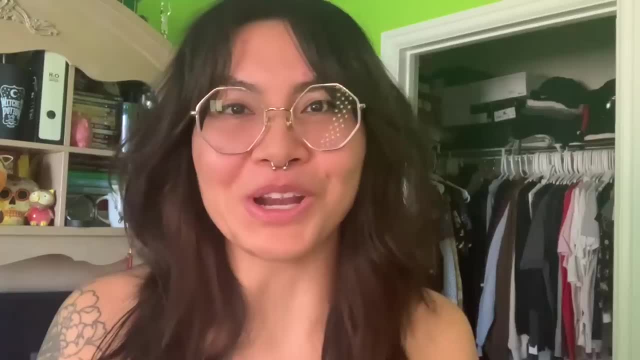 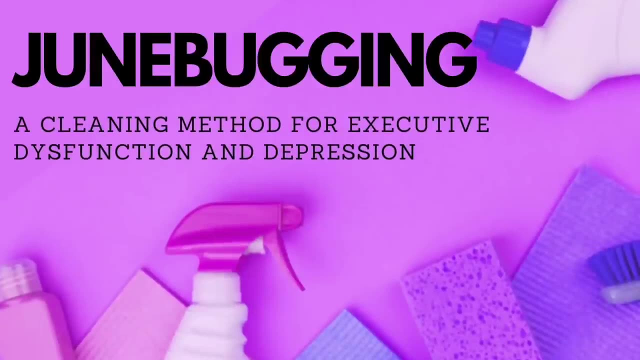 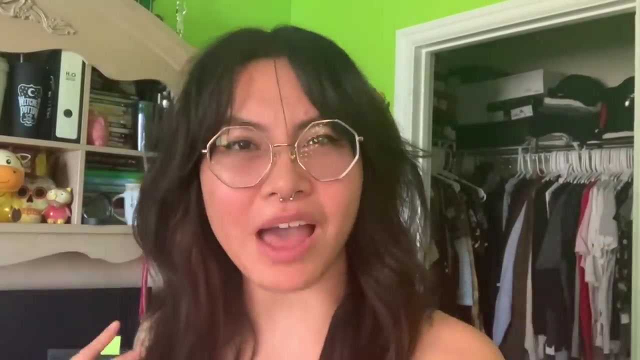 with thus avoiding the problem and making it even worse. Hi, I'm Cassie. Hey, Hi, Hello. I hope you guys are doing good. I hope you guys are having a great day, feeling well, thinking great thoughts, and if you're not, maybe you should clean your room. 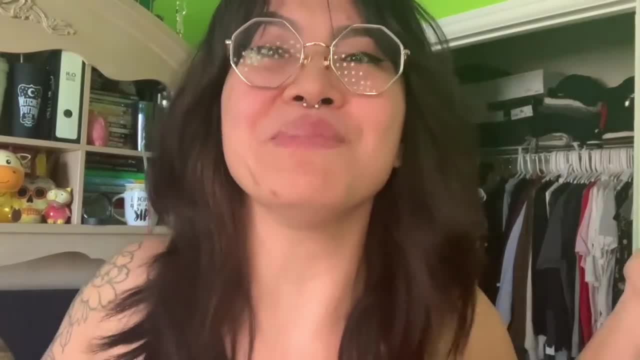 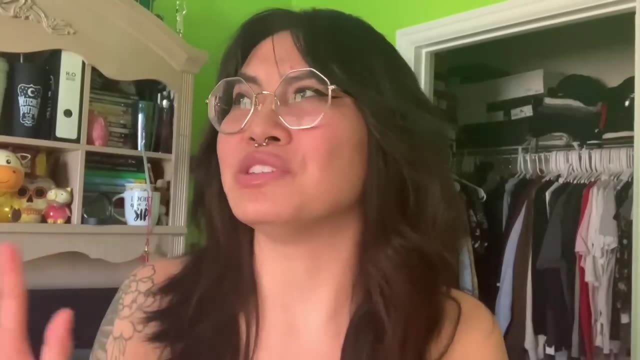 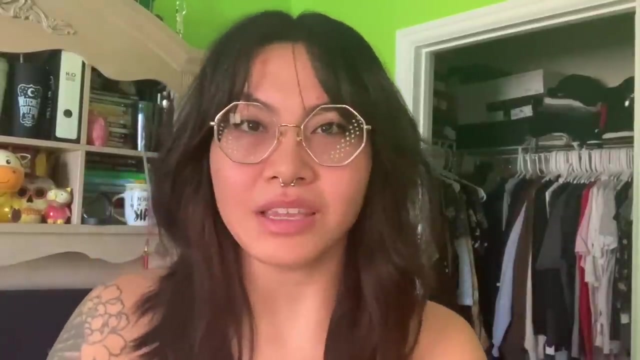 If I called you out, I really didn't mean to call you out because we're gonna be cleaning together, because girl, boy, demon, I don't know. Please, demons, no, you're not welcome here, But we're in this together, like I said, and I find that when my room is clean, 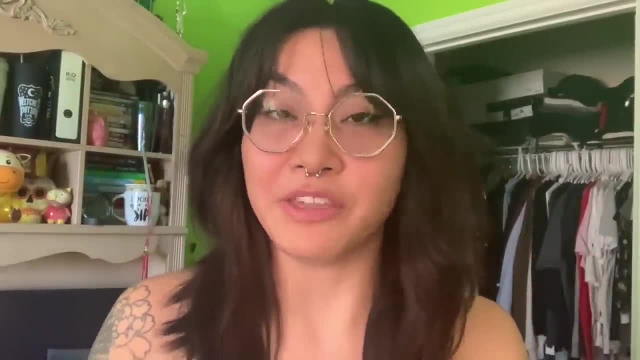 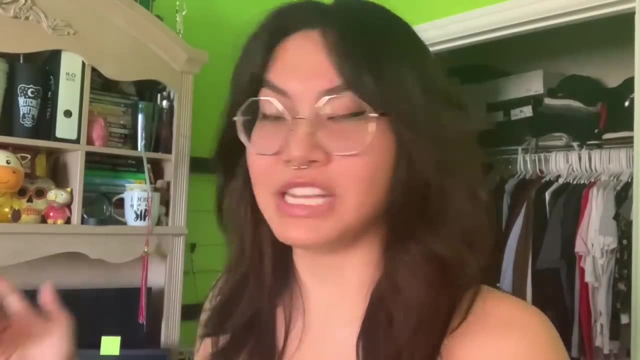 I'm feeling good. I typically only ever clean my room when I'm either feeling the lowest of the low or coming out of the low and feeling the highest of the highs. and I decided I would take you guys along with the spring cleaning of my room. I'm going to show you guys my room- kind of personal. 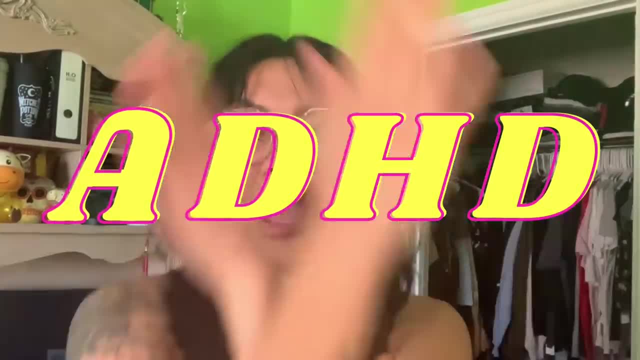 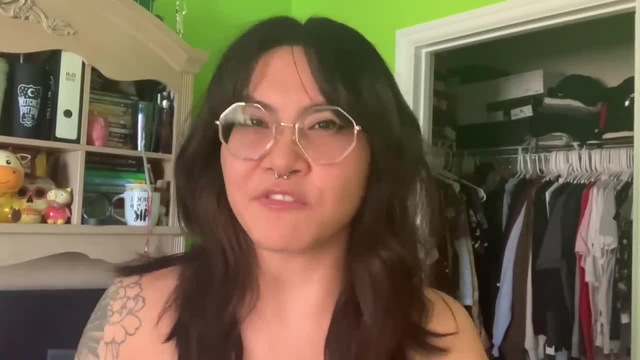 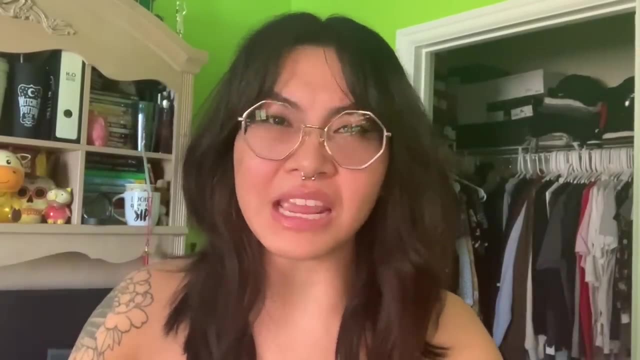 ADHD and cleaning are not the same thing, but I know historically ADHD and cleaning do not make ADHD and cleaning do not make the best partners. They're more like frenemies. So I wanted to share with you guys today a cleaning technique that has worked amazingly for me. but I've also learned. 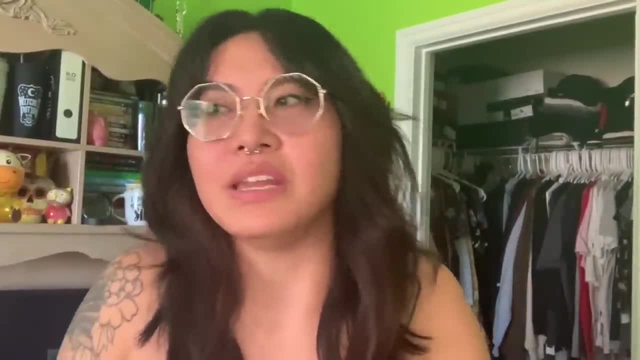 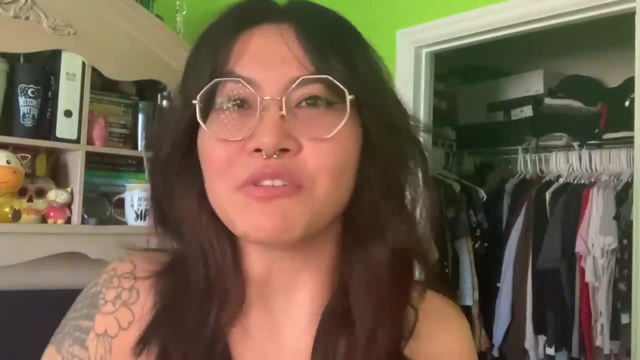 that this technique is what people with ADHD, autism and people struggling with depression use, and I just was like what? There's a term for what I've been doing and it's been proving great for me. This is so freaking rad, So this message is called Junebugging. 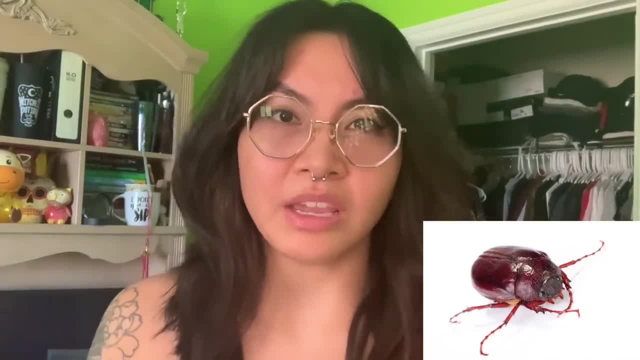 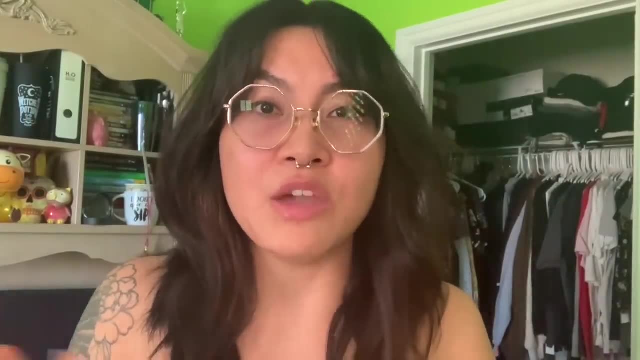 The Junebugging is based off of this insect, the Junebug that will go on to your window and literally look for holes to get into your home And it will try all of the entire window until it finds the perfect hole to get into your house. It's like dude, I need air. 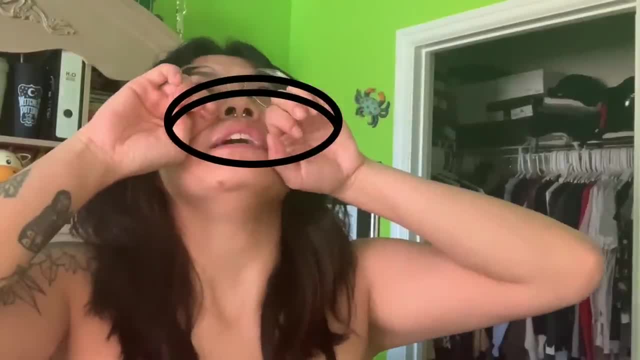 conditioning. Come on, Come on, man. Hey man, I need some of that air conditioning. Can you let me in, please, please? That's what I just think of. So yeah, as Junebugs do, that's what we will. 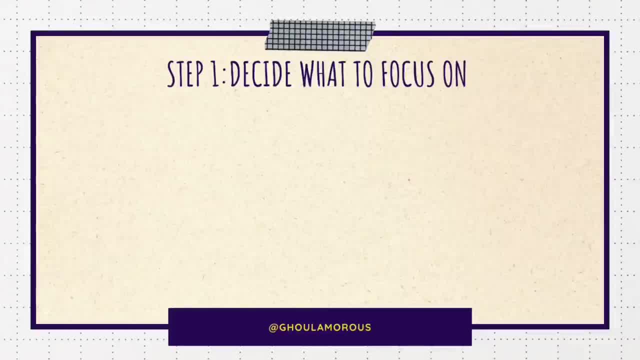 do And we're going to focus on one thing at a time. By focusing on one thing, we're not going to focus on: okay, I'm going to do the bed, I'm going to do the laundry, I'm going to do the. 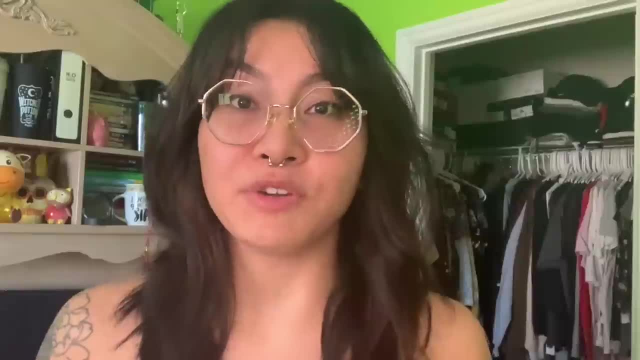 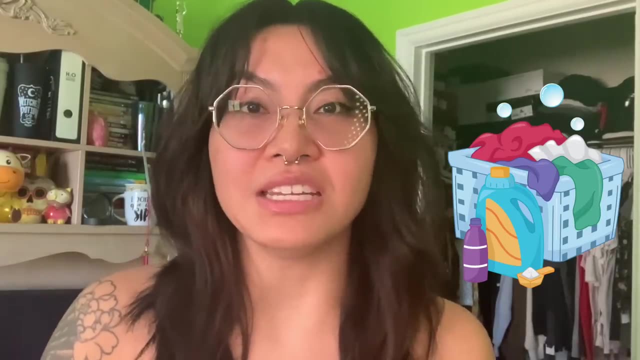 bedroom, or, okay, I'm going to do the bathroom. You are going to focus on one specific thing: in your bedroom, in your bathroom, I'm going to clean the toilet. I'm going to get one load of laundry done today. I'm going to clean out my dresser, clean out my closet- If you have a walk-in closet. 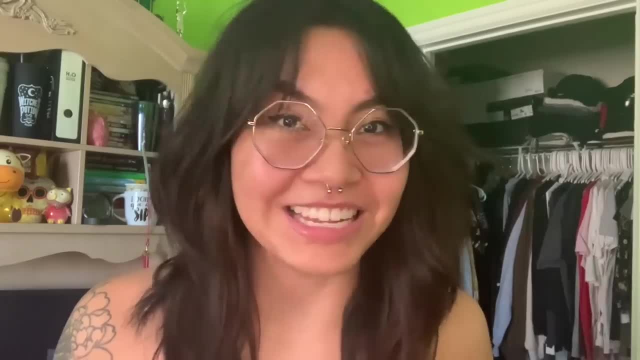 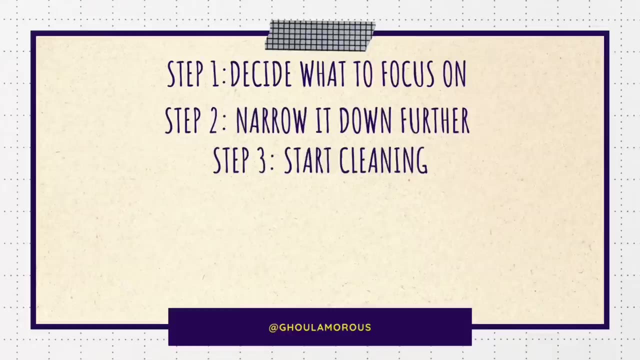 it could be a whole lot. So what you would want to do in that instance is: I'm going to focus on my shirts in the closet, I'm going to focus on my pants in the closet, my shoes And, once you've made a decision, go ahead and start cleaning. But the main benefit of a clean room, 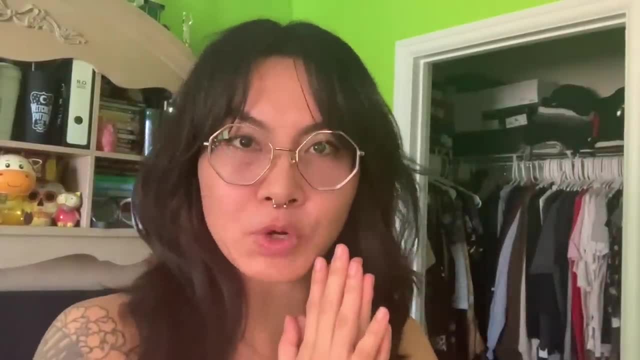 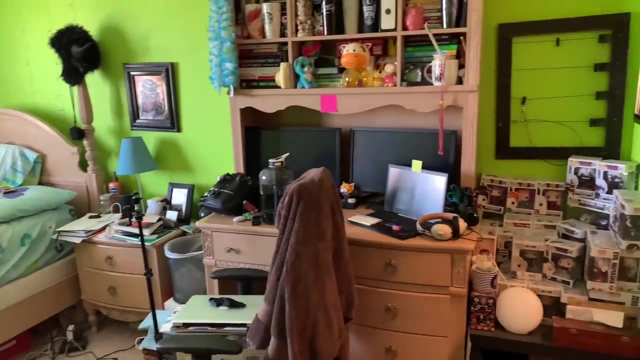 is feeling good, So why don't I take you around my room as if you were shopping around for a new fucking home? So this is my room. It's not the best it's been, but it's also not the worst it's been. 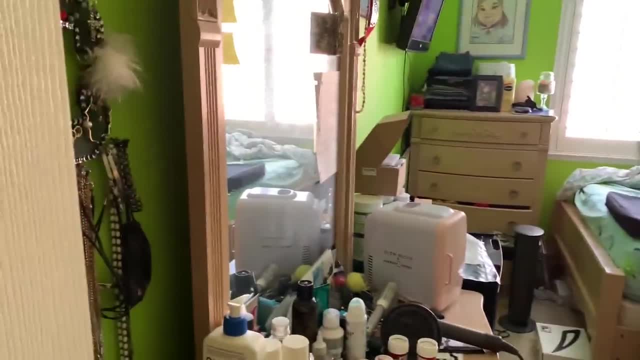 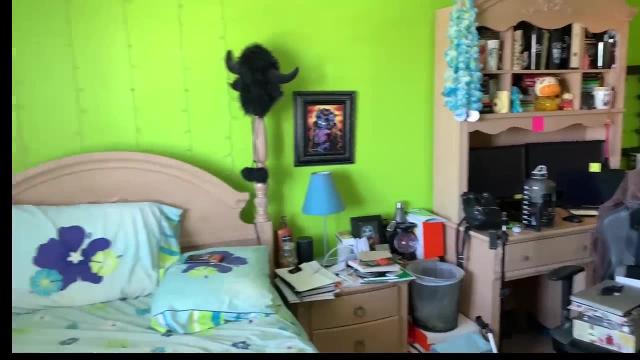 I at least have some walking space, so that's a plus. This is my childhood room, so that's why the color is loud and the decor is all over the place, But it's cool to know that these all still make up me. Also, thank you to my mom and dad. I'm forever grateful to know I always have a home. I 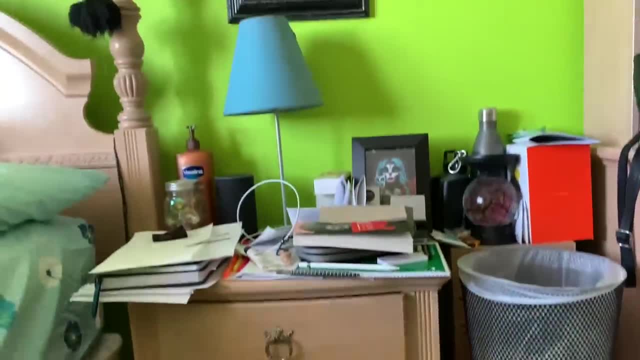 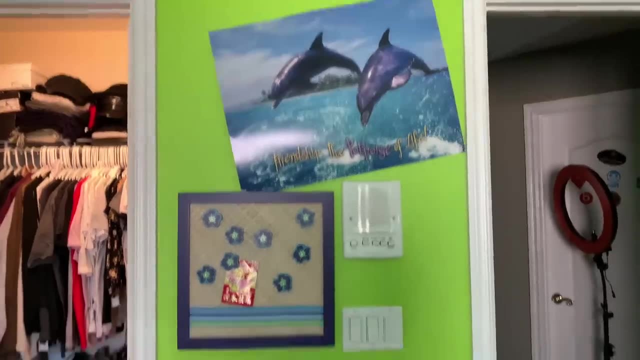 can come back to should anything go wrong in my life, like now. I love you. Oh, and this is my designated chair, where everything goes, as you guys may have seen in my intro video, And I have a little ghost story about that poster, if you want to stay till the end. 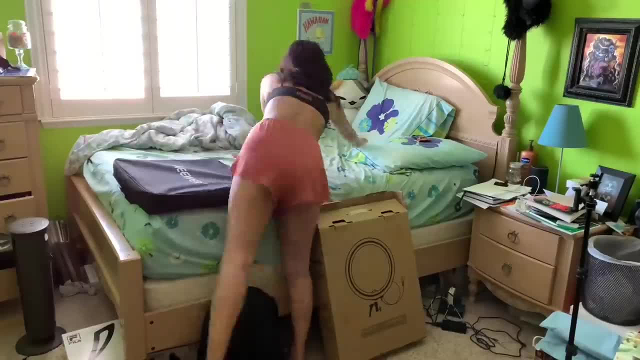 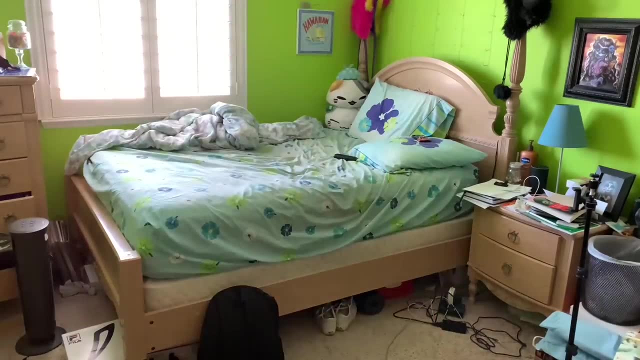 for that. First off, sorry about my fit. I live in Las Vegas and it'd be so hot and I honestly totally forgot to change my attire for this video. I just went straight into it. But I am focusing on my bed. I chose my bed so that way I can do the laundry while I'm working on everything else. 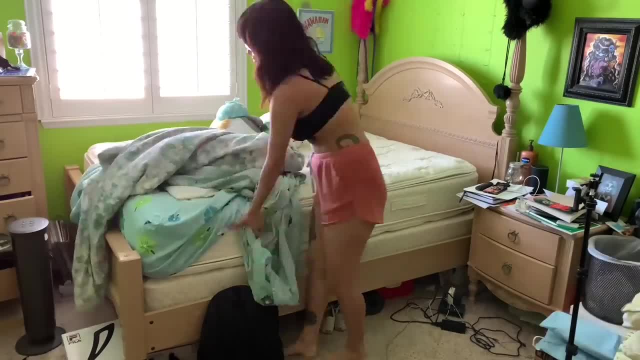 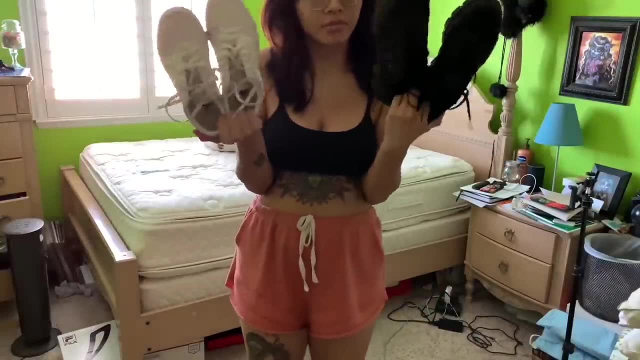 around my bed and making my way through my room, I figure: why not hit two birds with one stone? I tend to leave my shoes everywhere, but since I'm strictly focusing on my bed, I'm putting my shoes where they need to go, so that way, when I get to that area, I can go ahead and put it away. 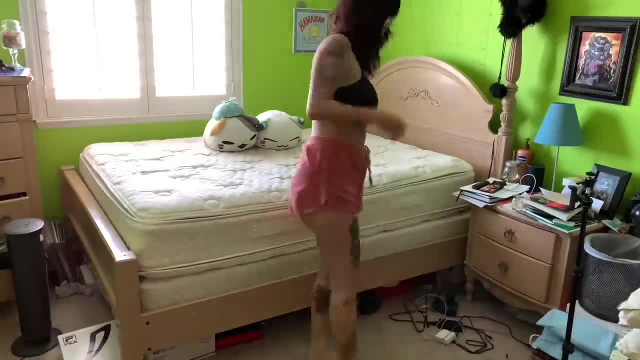 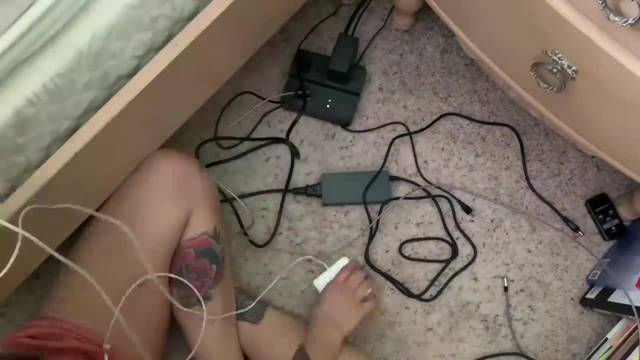 unless it's real quick to go ahead and put away, then do so. But again, we're still focusing on one thing at a time. Since I finished focusing on my bed, I am moving on to the next thing, which are my cords. 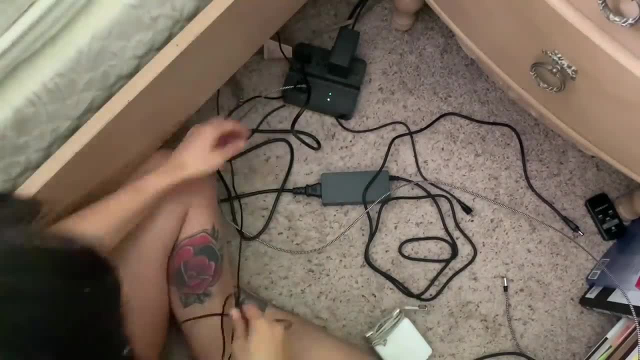 I like to work clockwise around my room because each area of my room is technically its own segment, and that's what I. I like to work clockwise around my room because each area of my room is technically its own segment and that's what I find every day. 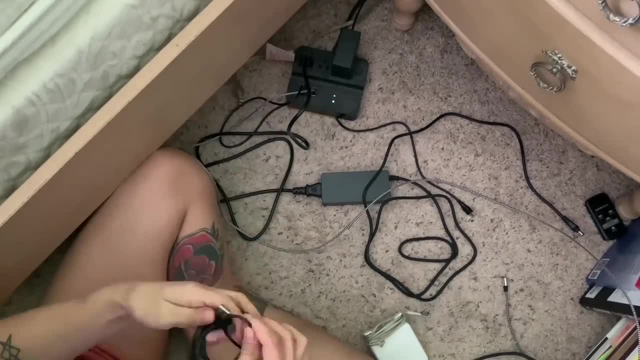 So I might as well do the laundry and sort things around my room for the rest of my life, But I'm interested in living there. I think this piece here was own segment and that's what I find helps me stay on task. Side note: you do not need to tackle. 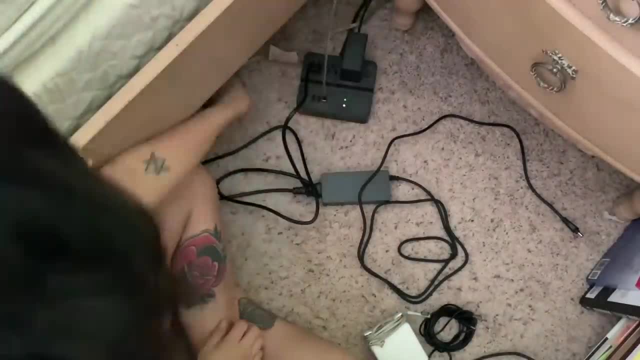 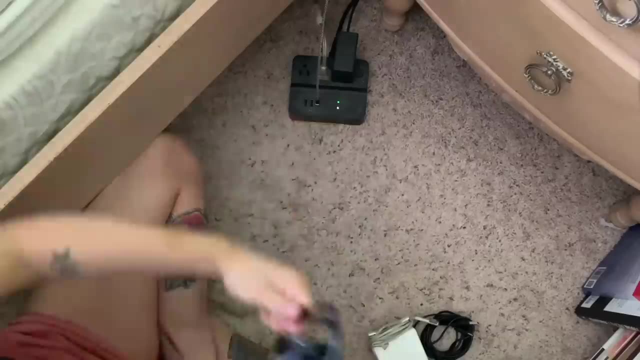 cleaning all in one day, like you see me doing here. It's okay to have it spread out or even use this technique as a way to maintain cleanliness after you have cleaned everything. So just wanted to let you guys know you do not need to follow the way I am doing it. 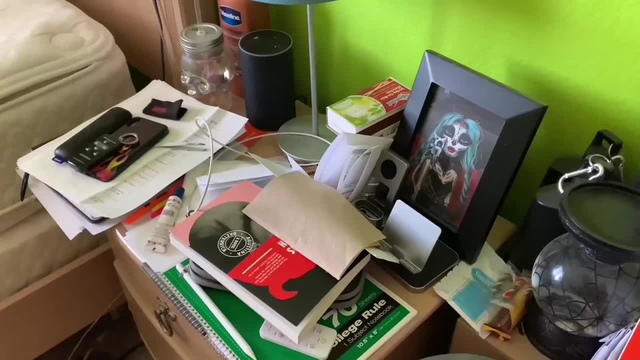 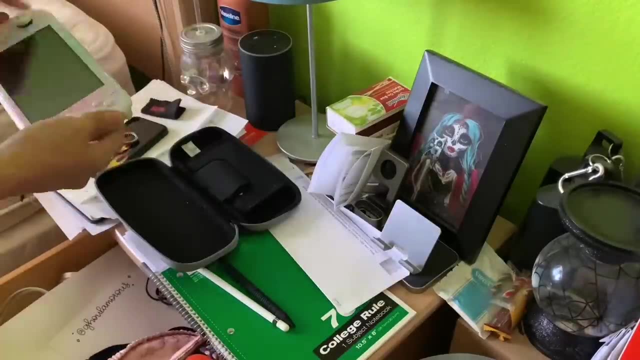 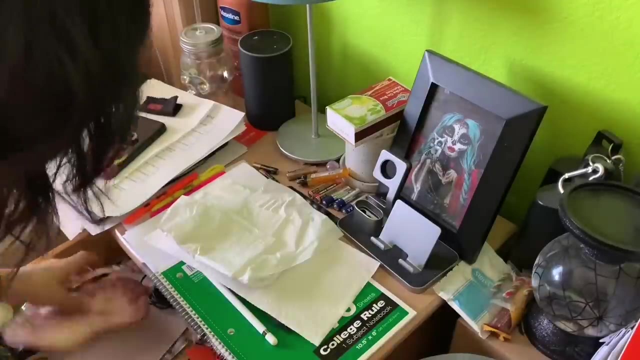 I just so happen to have the time and energy to get it all done today. Oh my god, my nightstand is a mess. Any and all things that I use will go there, and although I'm the worst at planning and journaling, I try my best. So that's why you see the handful of notebooks and everything. 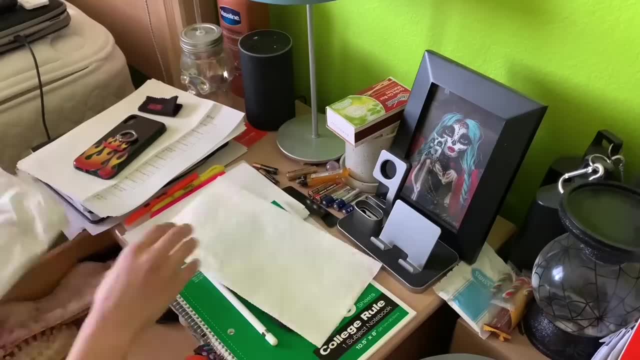 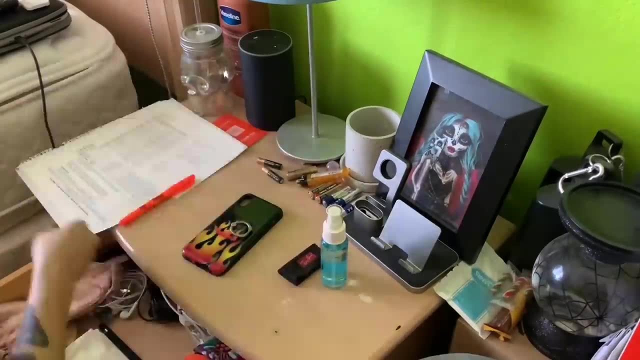 Oh my gosh, Now you see me organizing my drawer. You actually do not necessarily need to do this. You can just put things in the drawer where they go and then come back to it later to do more of a deep clean. But I figured, while I have the time, why not? 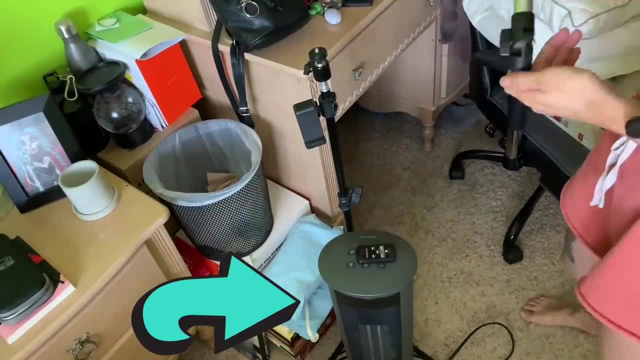 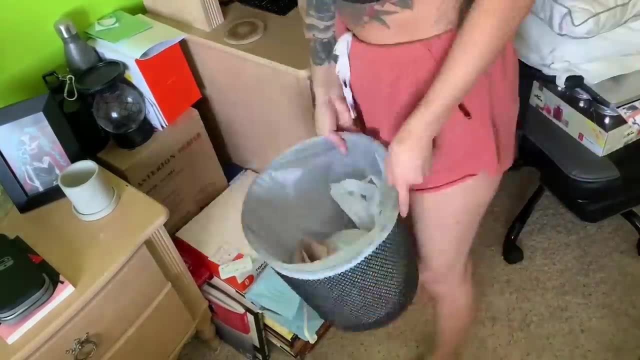 Oh, look, more shoes. I don't know if you guys saw, but that heater used to be by the foot of my bed. I moved it to this area to put it away in the brown box behind my trash bin to stay focused on the bed, while also having the visual reminder to put it away once I get to that section Also. 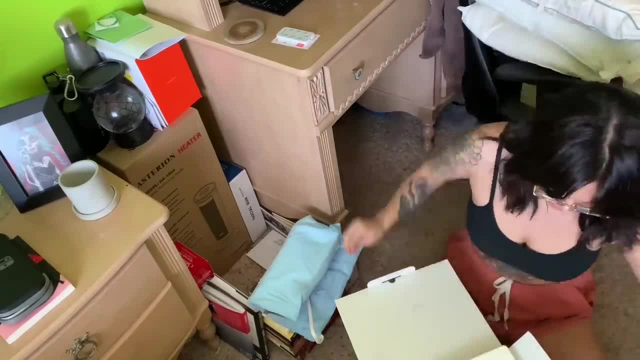 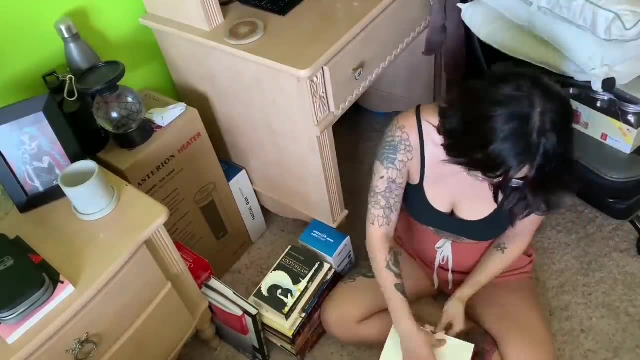 I like to keep the boxes for storage, warranties and preserving their condition when not in use or moving. You don't have to do this, but I find that this is easier for me to see where my stuff is, while maintaining some organization in my room. 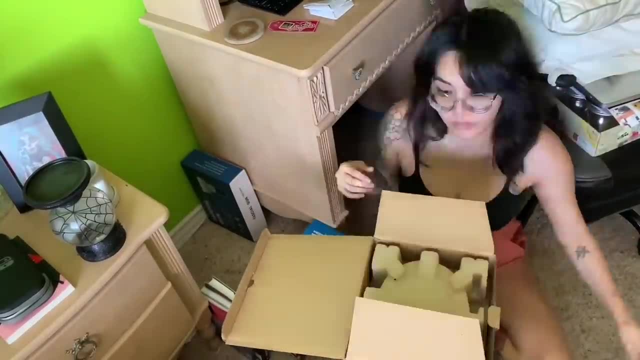 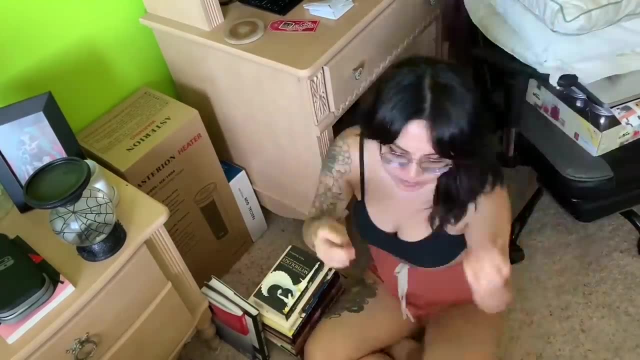 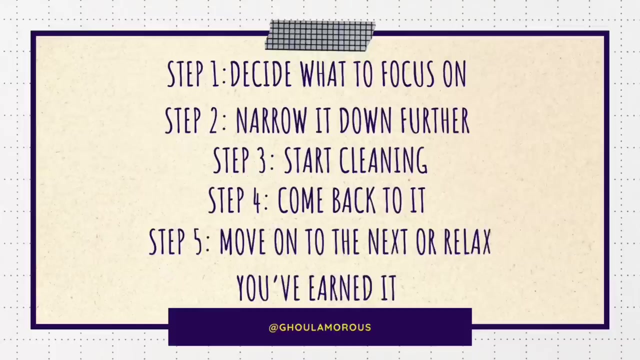 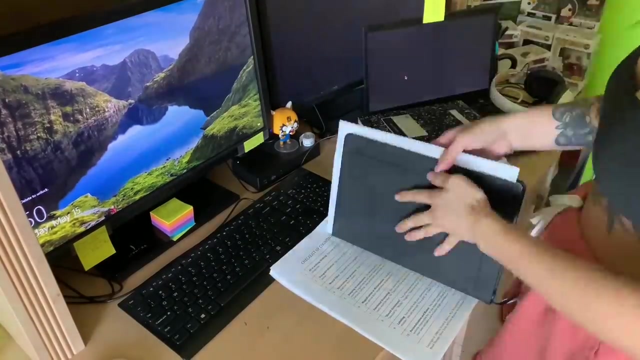 Remember, it's okay to take breaks so long as you come back to Junebugging to finish the section or take the break after you've completed your chosen section. You've earned it after all. Oh, looky, more planners and journals. I ended up placing a few by my bed because there's a planner. 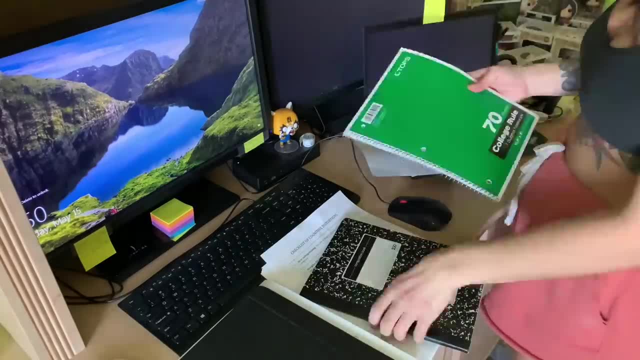 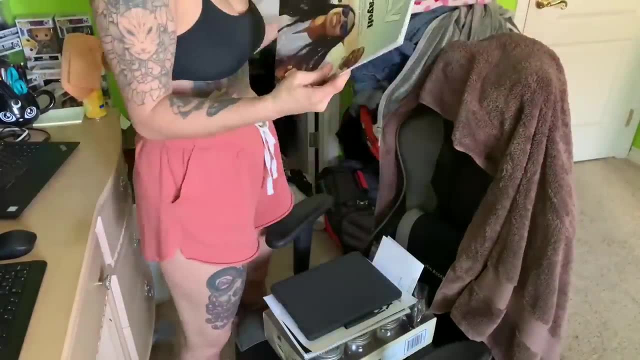 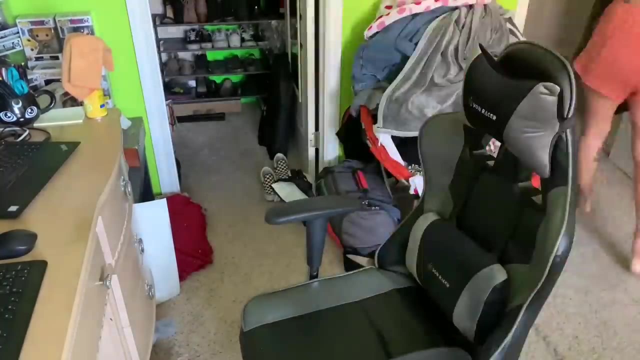 and a journal I do use quite frequently, but place the others that I don't use in the drawer and recycle pages that were no longer in use. Now, I know clothes are one of the easiest things to put away, but this is my safe clutter. 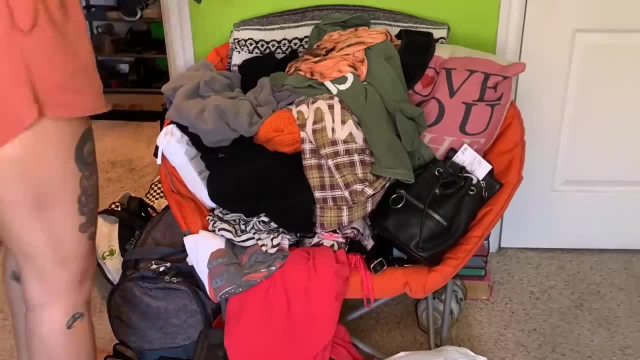 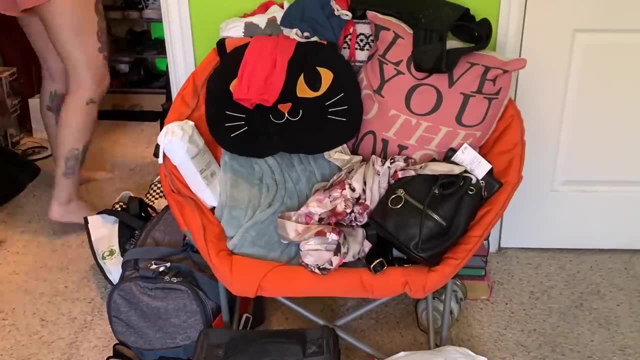 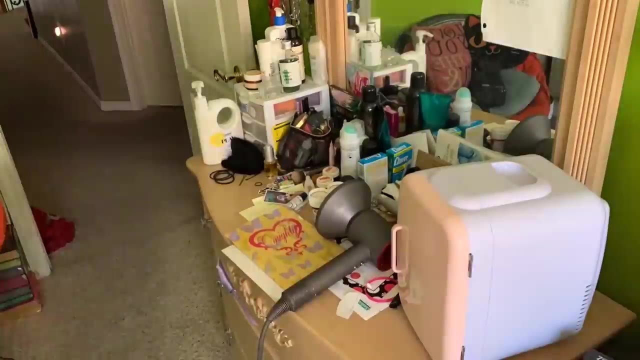 meaning I don't mind it staying this way. it doesn't necessarily affect me and I know where these items are at all times, But since my entire room is going to be clean, my safe clutter is no exception. Since my brothers have moved out of the house, I have the bathroom all to myself, But since I'm 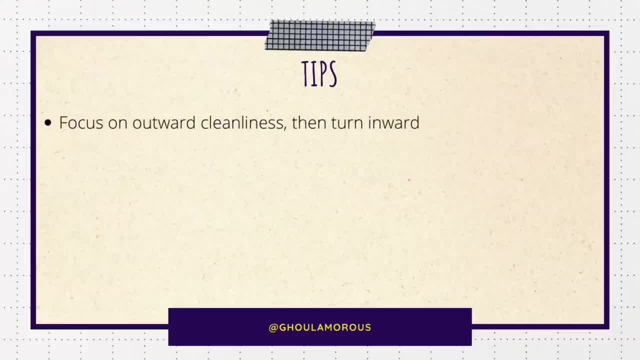 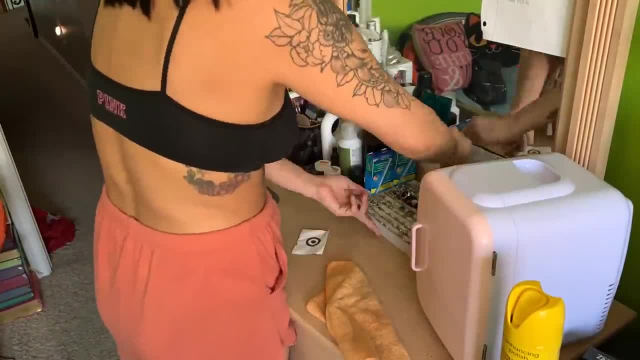 focused on just cleaning the outward appearance and having things in their areas. for now. I'll be doing the deep cleaning tomorrow of reorganizing my drawers and moving and throwing away things that I no longer need in my vanity, Also keeping the items I use religiously on the top. But for 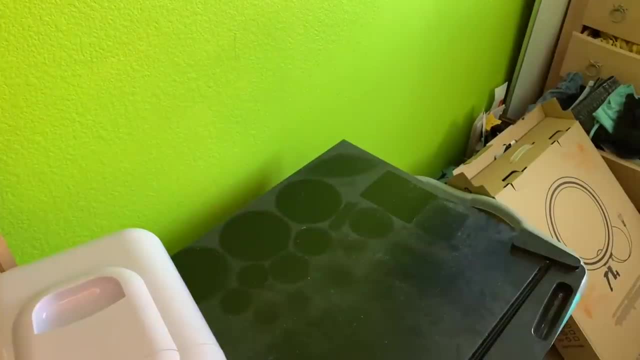 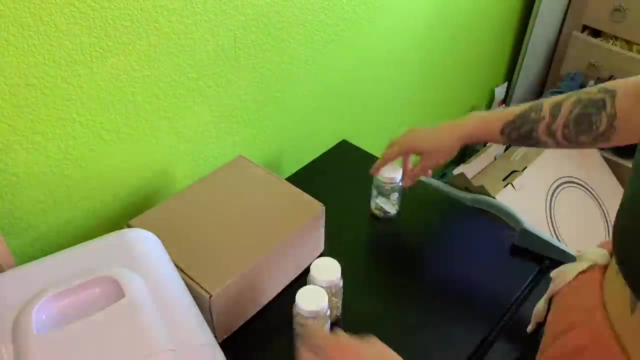 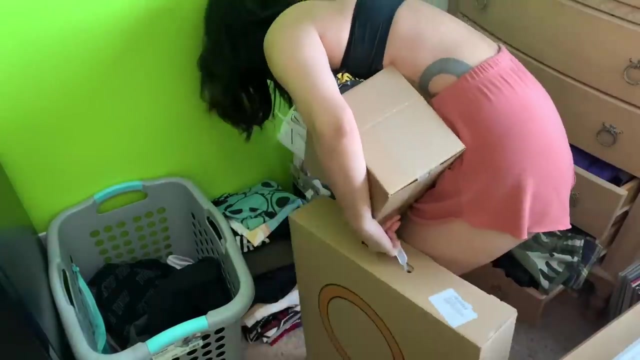 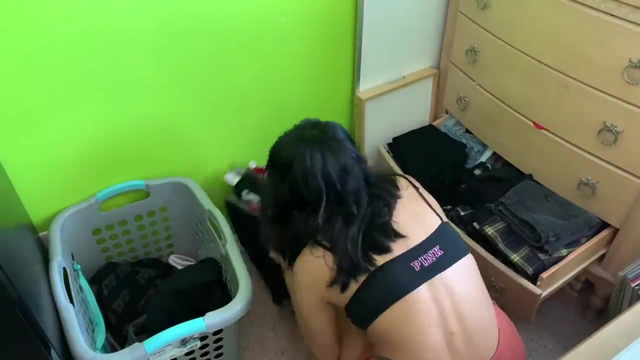 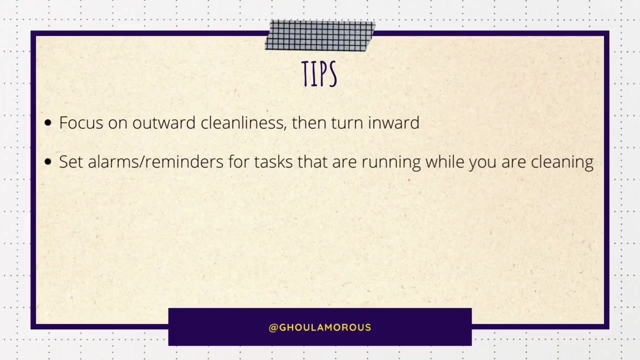 now just focusing on the visual cleanliness before moving inwards. Here's a tip: Set an alarm timer or reminder with your smart devices to check on other tasks that are running in the background. Here's a tip: Set an alarm timer or reminder with your smart devices to check on other tasks that are running in the background. 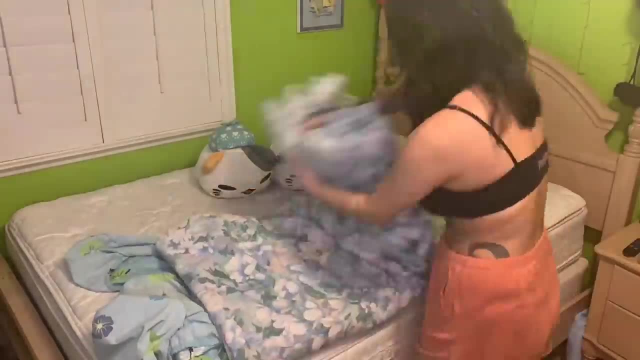 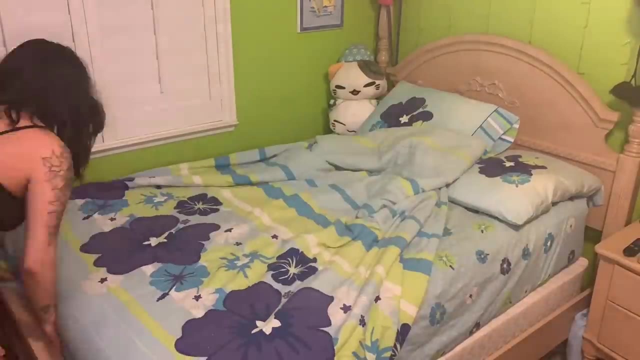 While you are June Bugging, I tend to forget about laundry, which is what happened here, and the alarms help. If your laundry is done, feel free to place it in its specific area so you can come back to finish it up, And here's the end result. 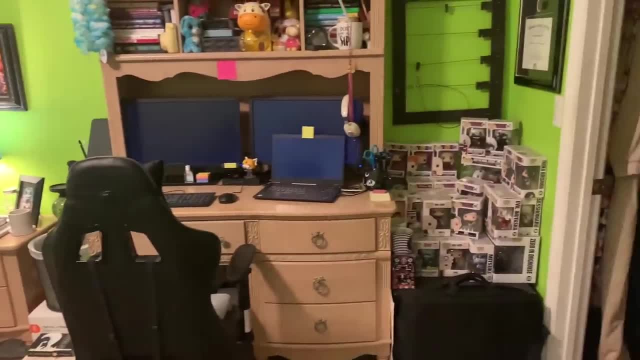 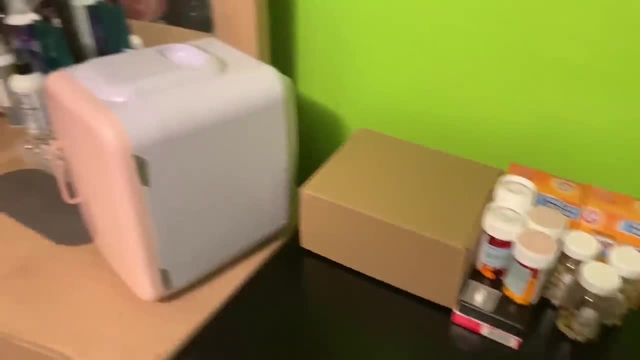 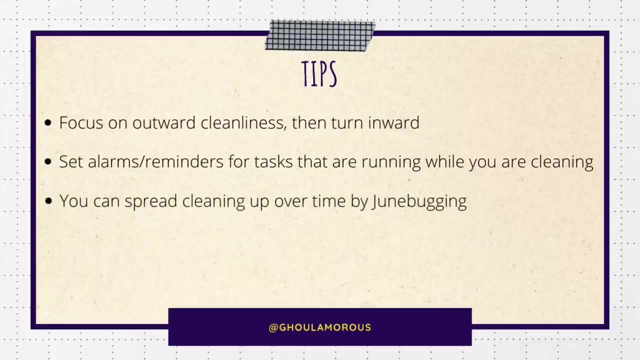 remember, you do not need to knock it all out in one day. it's okay to tidy up one day at a time, each section at a time, but if you did happen to clean everything, congrats. you can use this method the same way to maintain cleanliness of your home by focusing on one section for each day. 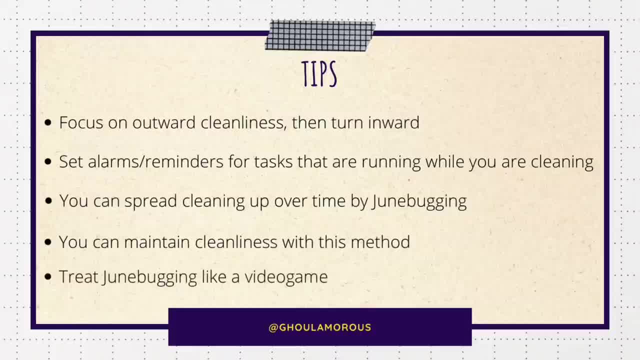 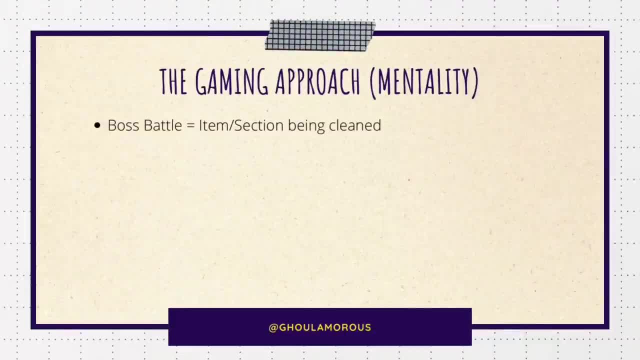 or if you're finding out that june bugging is still not working for you. think of it as if you were playing a video game or reading a book. i use the video game mentality by viewing the specific section as a boss battle. i can't move forward until i beat this boss. however, if there are items,